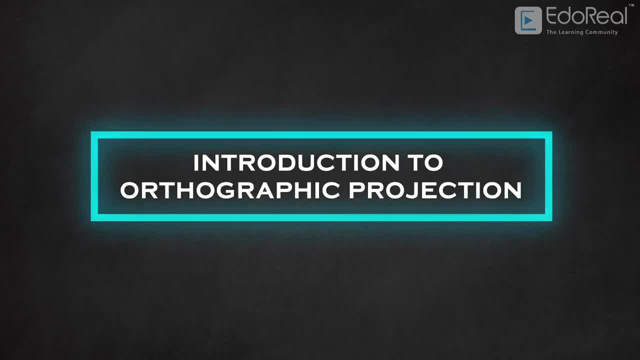 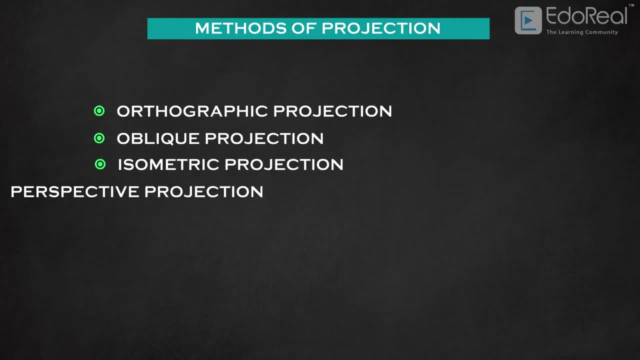 In this video we will discuss introduction to orthographic projection In engineering drawing. commonly, four methods of projections are used: Orthographic projection, oblique projection, isometric projection and perspective projection. First let's look into orthographic projection for now. 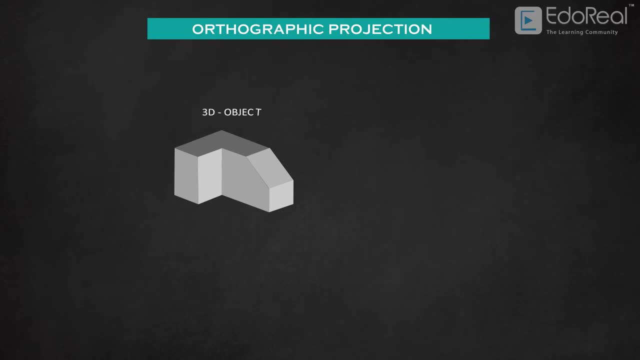 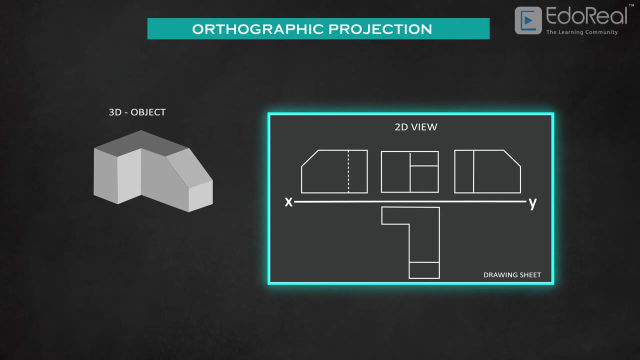 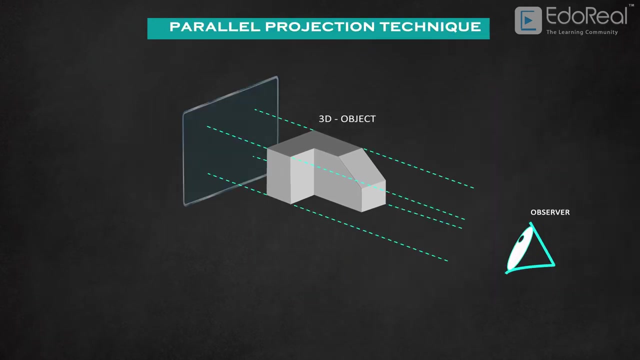 Orthographic projection means the representation of three-dimensional objects into two-dimensional views on the drawing sheet. We get these two-dimensional shapes using parallel projection technique. In parallel projection we project rays or line of sight onto the object. that produces two-dimensional shapes on the screen or projection plane placed behind the object. 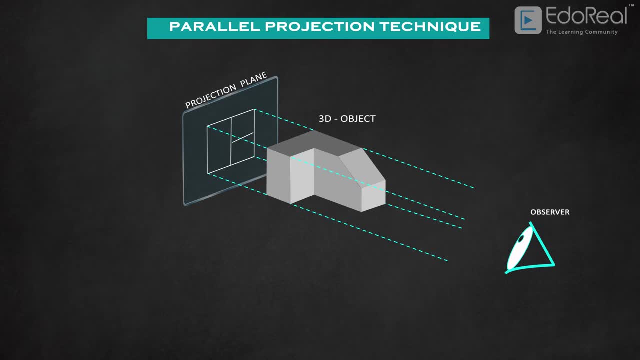 Parallel projection literally means line of sight or projection lines are parallel to each other. These projection lines are projected perpendicular to the plane. So if the projection lines are parallel to each other and also perpendicular to the projection plane, it is called orthographic projection. 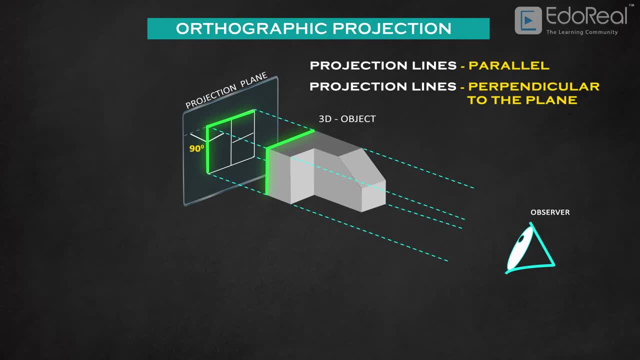 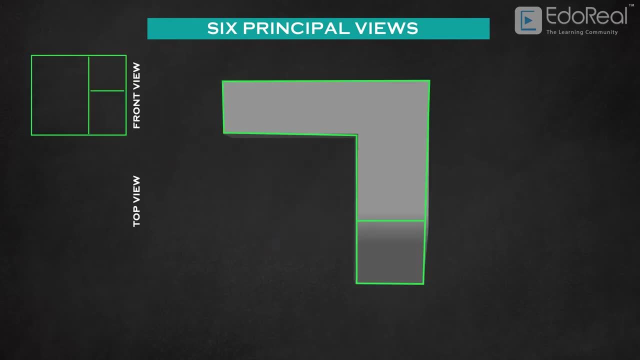 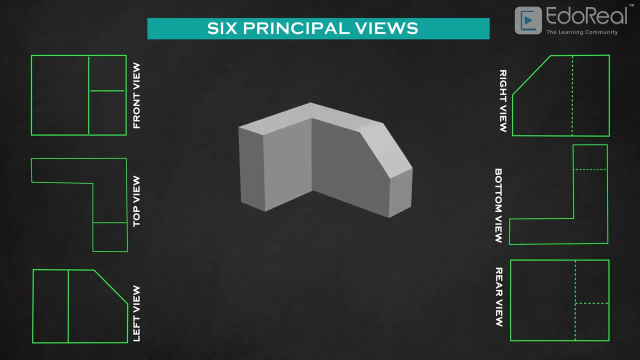 By this projection, the true dimensions of the object will be preserved. Every three-dimensional object contains six sides: front side, top side, left side, right side, bottom side and back side. So six views are possible for a three-dimensional object. 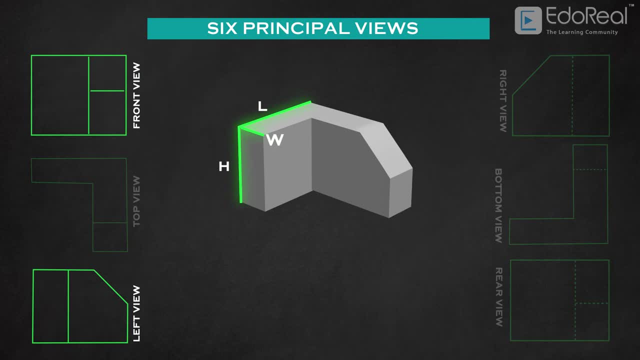 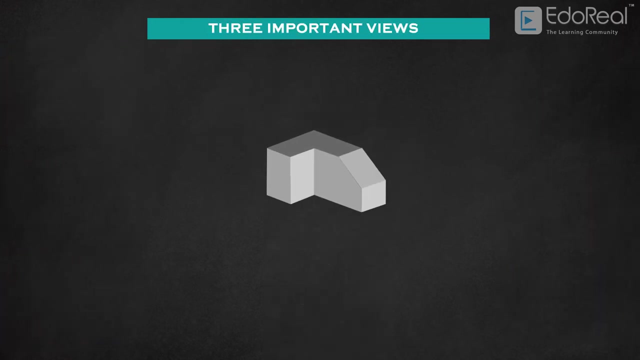 From these six views, at least two views are required to represent complete dimensions of the given 3D object, like length, width, height. Sometimes it may require three views. if it is a complex shape, Three views are important among six views. We can represent any object using these three views. 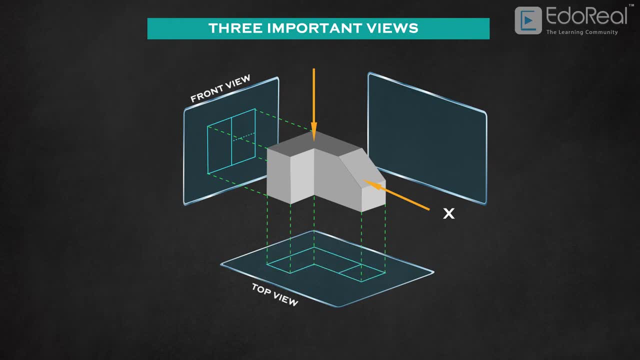 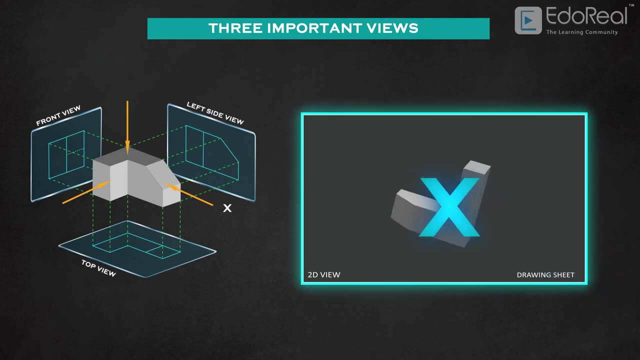 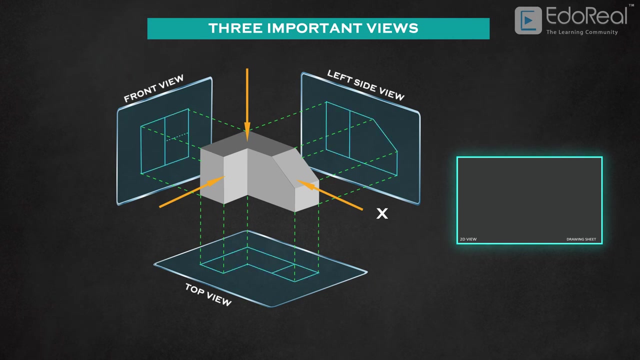 They are front view, top view and side view. We take these three views because we cannot draw three-dimensional complex objects on paper, So we convert it into two-dimensional shapes and draw them on paper. Generally, we follow a format to represent the three views of an object on a drawing sheet. 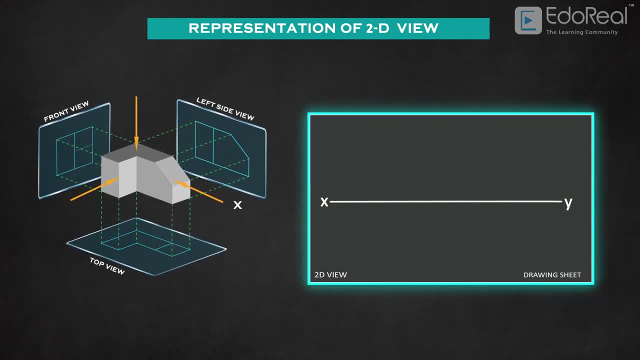 We first draw a reference line on the drawing sheet. The front view of the object is drawn above the reference line. The front view of the object is drawn above the reference line. The front view of the object is drawn above the reference line. The top view is drawn below the reference line.